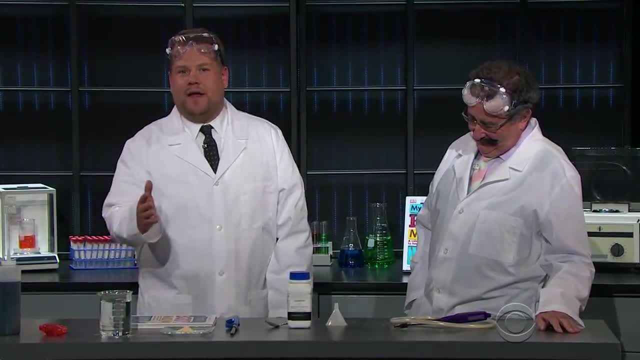 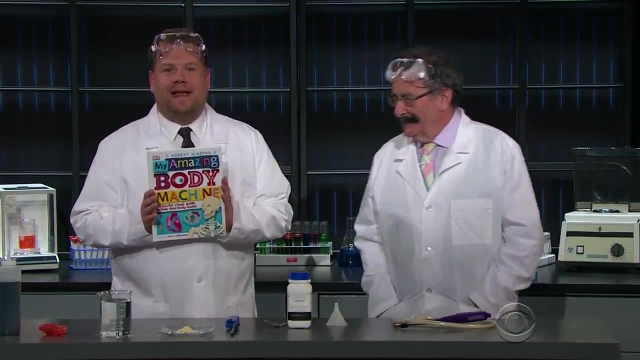 Our next guest is Professor of Science and Society at the Imperial College in London. He holds 23 honorary doctorates and is the author of this brilliant new book, My Amazing Body Machine. Please welcome our good friend, Professor, the Lord Robert Winston. 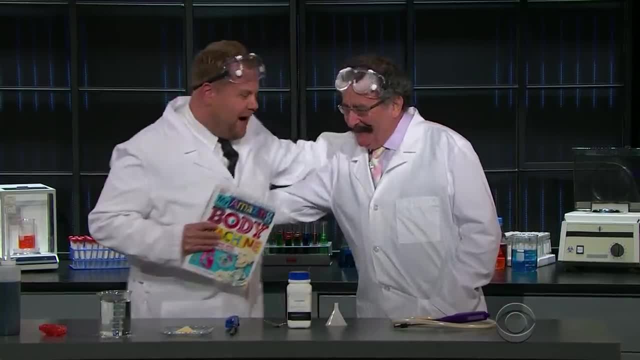 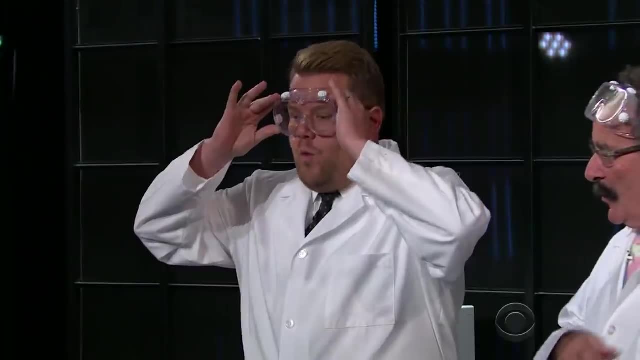 Thank you for coming back to see us. We love it when you stop by. All right, so, Robert, we are ready. We're in the zone. Let's get our science on. What are we going to be doing first? Let's start with the thing at the end. 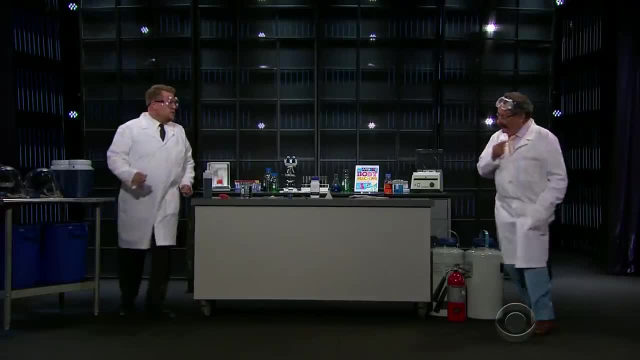 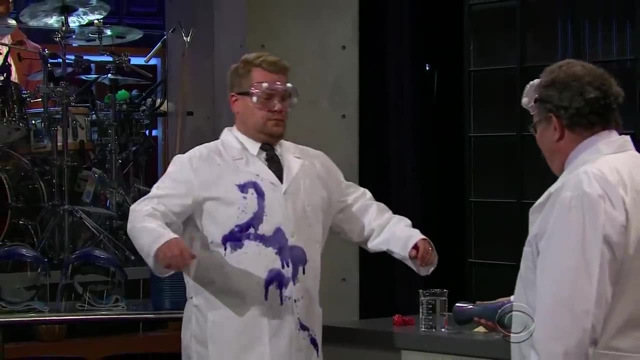 With this We'll come round, yeah, OK. So basically you've got quite a smart white coat on. Yes, Well, I'm a scientist, that's what I do. It's too smart. What, Robert? What is? 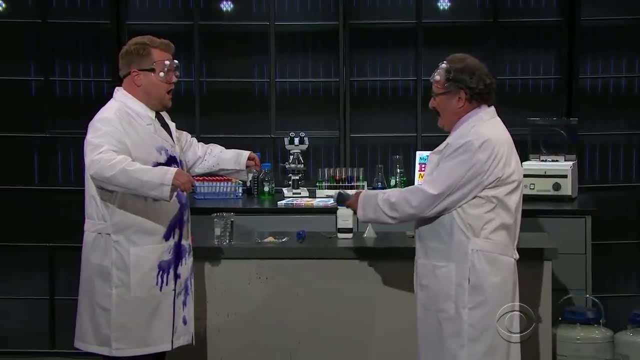 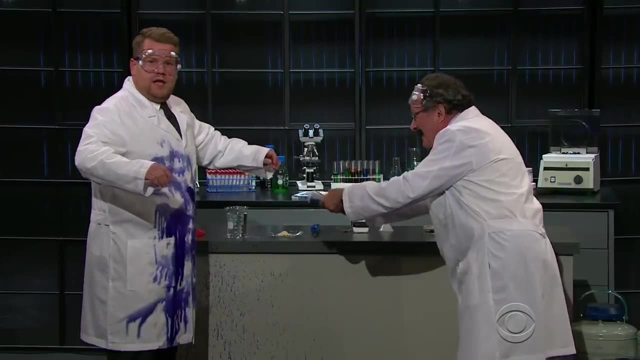 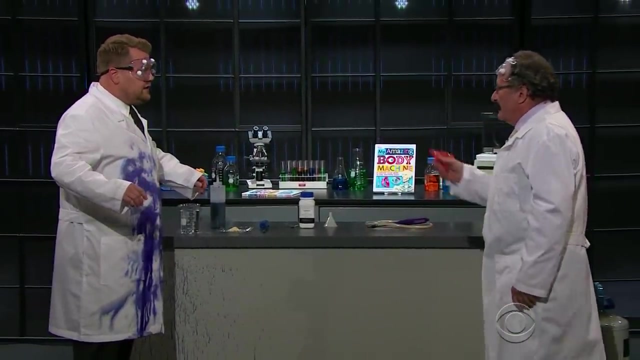 Let's get you a bit bluer. That suit isn't worth anything, is it? Well it's, It's worth a little bit. yeah, This is a solution to dry cleaning, Right? So that was. This is alkali, OK OK. 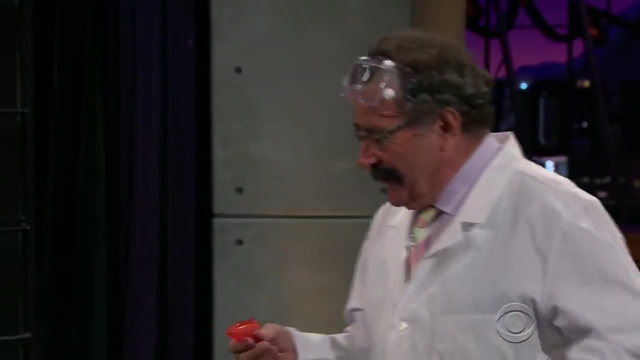 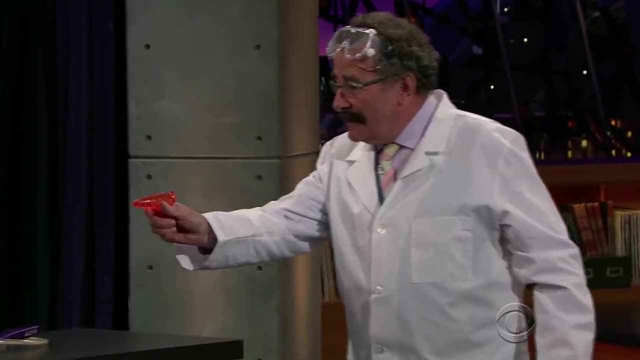 And the alkali is blue? Yeah, Because it's got a blue dye in it. OK, And what we're going to do is to squirt you with acid to neutralise the alkali. Wait, hang on. What do you mean? 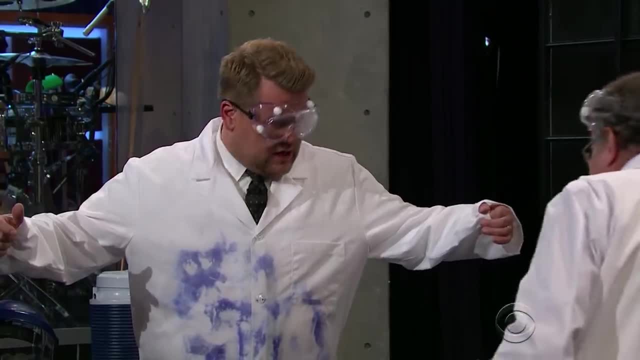 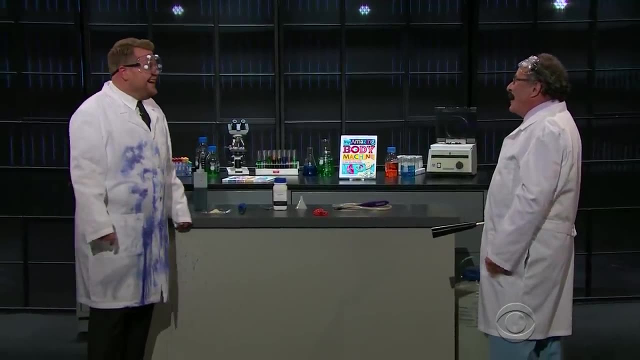 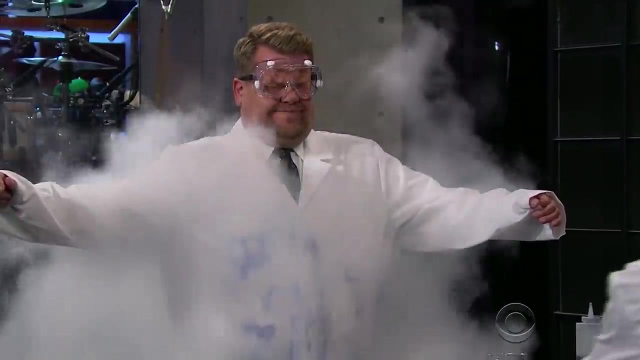 It's going to take ages. Look at that, Look And then it Look. it's rubbish. This is carbon dioxide, so carbonic acid. Carbonic acid actually is much more effective. OK, Let me stand well back Just a moment, please. 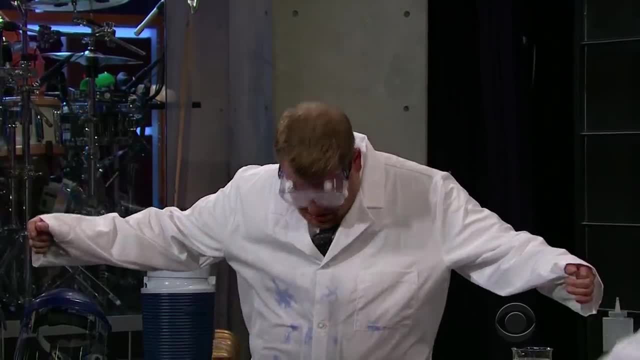 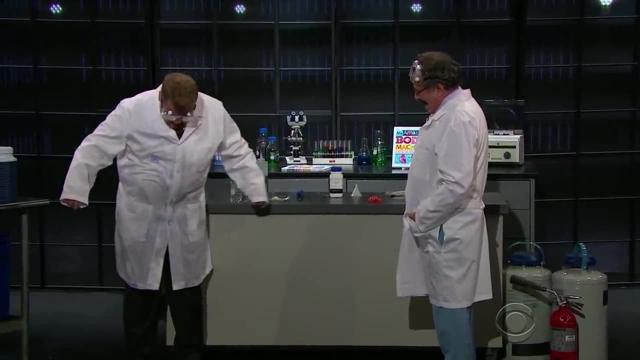 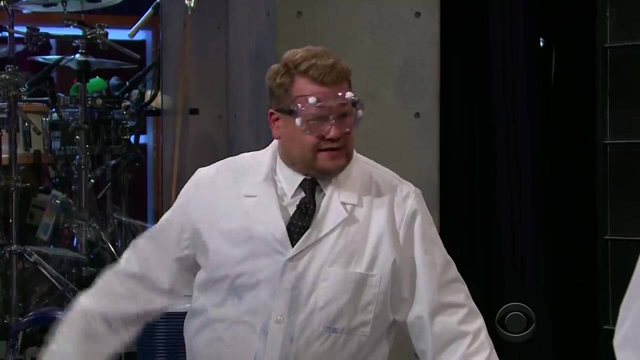 Now wait for the reaction. Look almost clean: CHEERING AND APPLAUSE. Right, I feel like this isn't even a science thing. you've just come up with some way to do that to me, But that's pretty incredible. that's amazing. 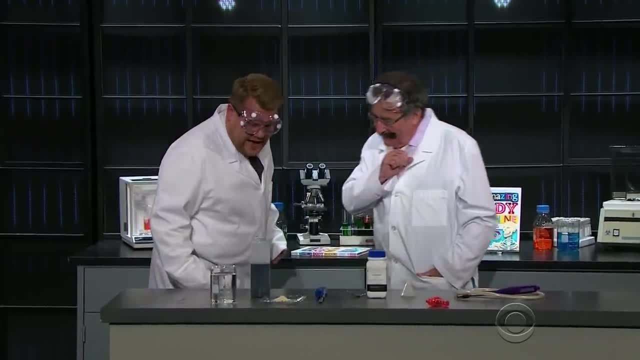 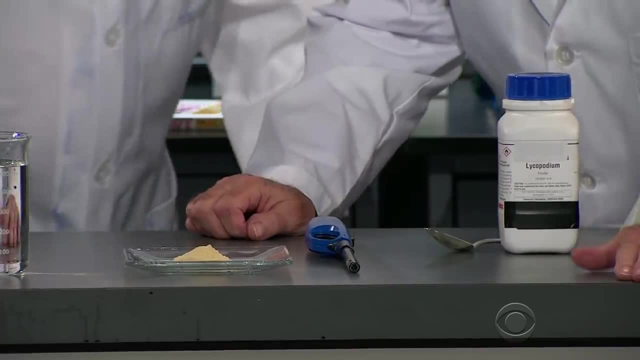 It's just gone. What? I'll give it that. What else have you got for us, Rob? What else are we going to do? Let me see, We've got this. Oh yeah, now what is that? That is lycopodium powder. OK. 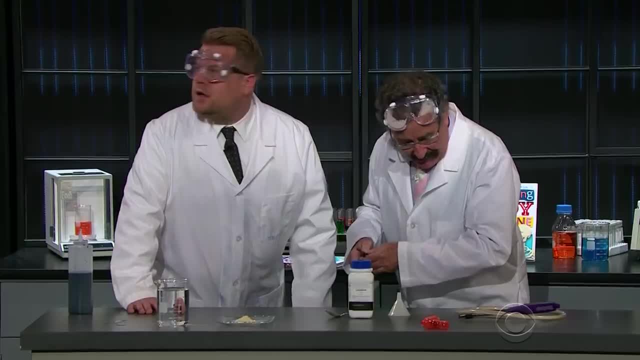 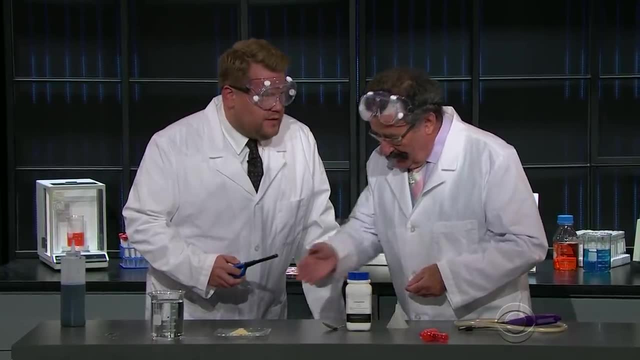 And it is quite explosive. so can you, Do you want to try lighting it? No, Go on LAUGHTER. When you say quite explosive, what do you mean? Try it and see On a scale of one to ten, how explosive is this Seven. 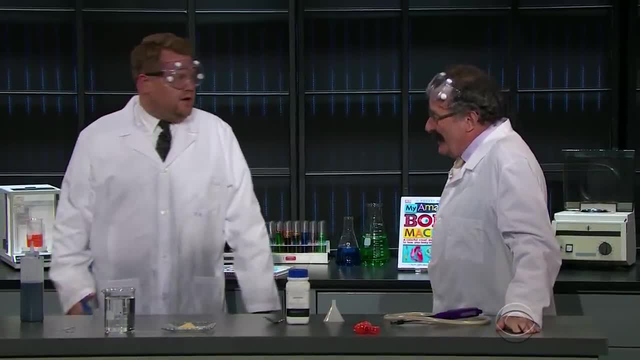 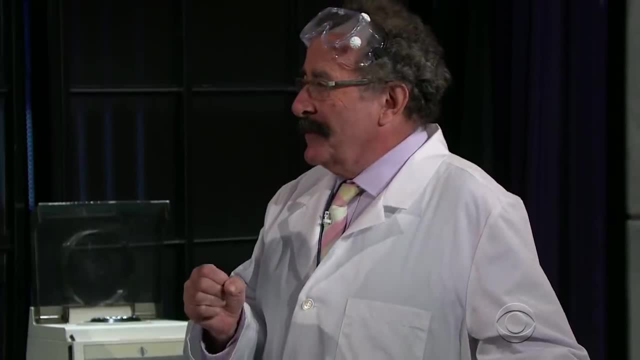 LAUGHTER. That feels a lot Right. These are. What am I doing? Just lighting this? These are exceptionally fine particles. They're about one thousandth of a millimetre across, OK, And they're all packed together. They come from a plant called lycopodium- Uh-huh. 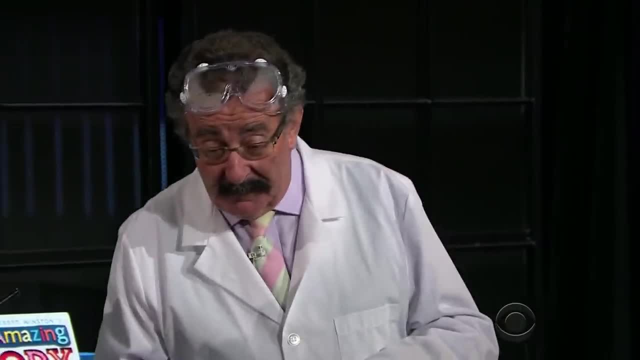 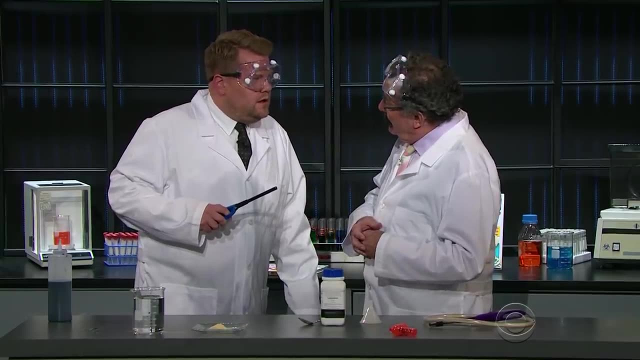 And it's a moss And it's used by all sorts of homeopathists to cure diarrhoea. It's supposed to be an aphrodisiac, but it also is explosive LAUGHTER. It's cured diarrhoea and is also an aphrodisiac. 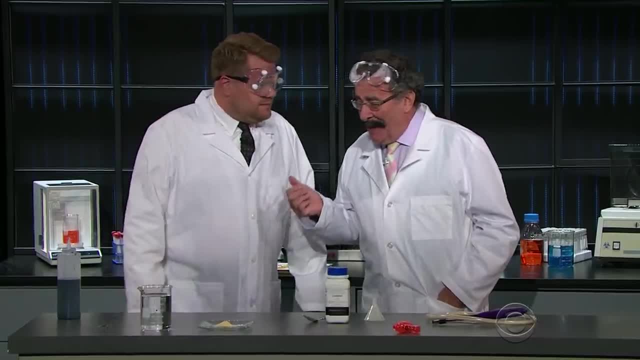 Very rare, Very rare combo that It is homeopathic, so it probably doesn't work, but it does explode, OK. So what happens? What's going to happen when I light this? Well, let's just have a look. 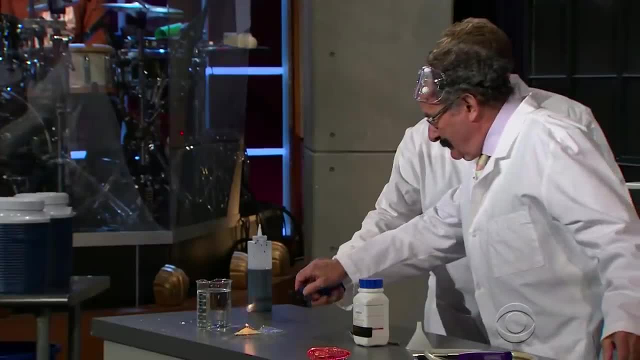 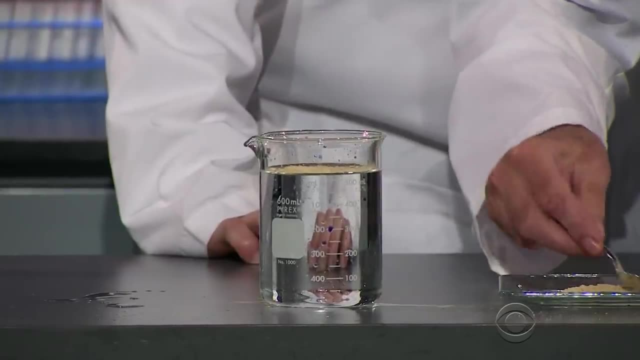 Not very impressive, is it LAUGHTER? What is that I mean? is that it? You see, it's a very fine powder. I'll show you how fine it is If we put it in this water. Yeah, put it in water. That'll set it on fire better, Robert. 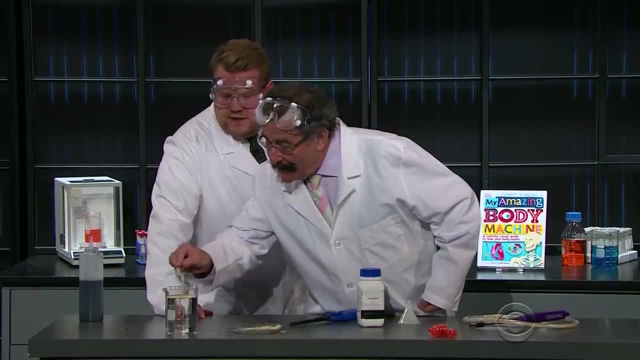 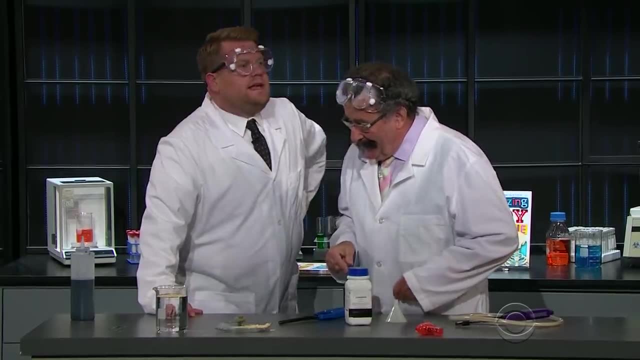 LAUGHTER. I mean, who's the scientist? It's hydrophobic, Now Right, And this isn't terribly poisonous. so if you put your finger through that dust, When you say terribly poisonous, I want it to be not poisonous or poisonous. 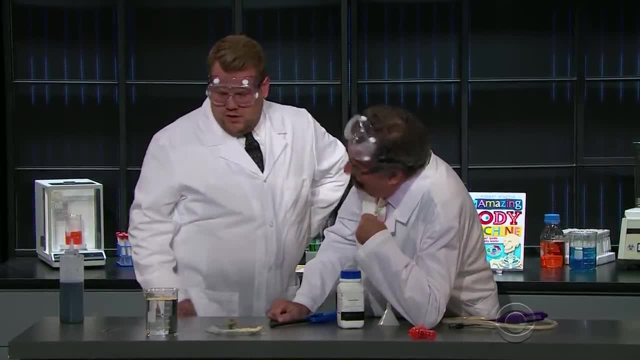 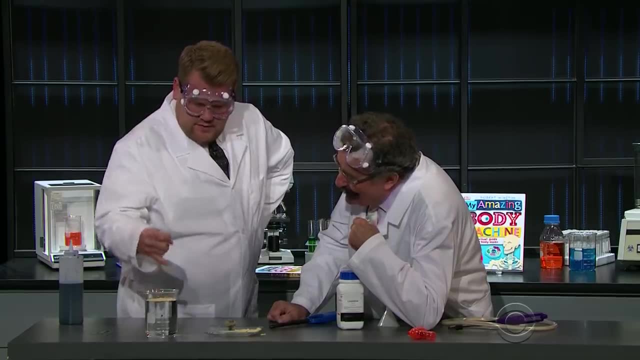 Put your finger in. Really. Yeah, Are you sure? Yes, Gently LAUGHTER, Uh, no, no, through the powder, not the water. What do you mean? Look Like that. Now look at my finger, Oh, look. 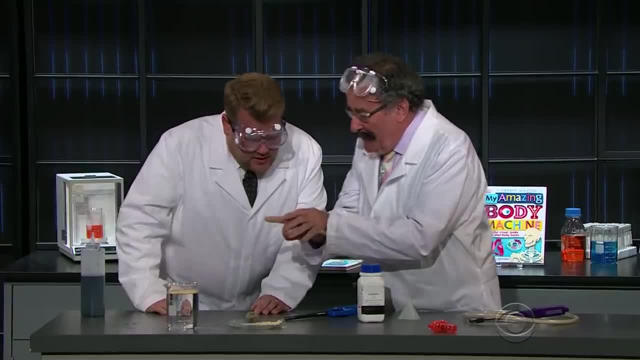 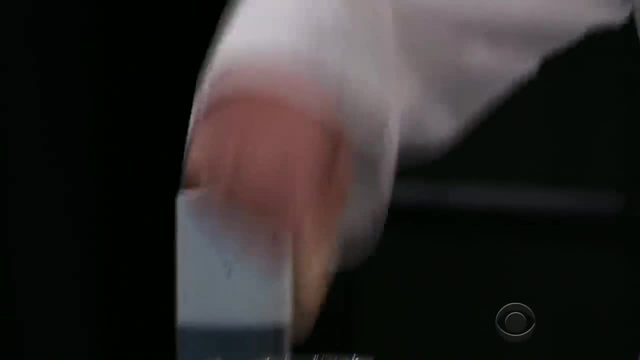 Oh, wow. So basically it's completely dry. Yeah, Because it's protecting my finger against the water because of the surface tension. Now, what we're going to do: we will make something a little bit more challenging, OK. 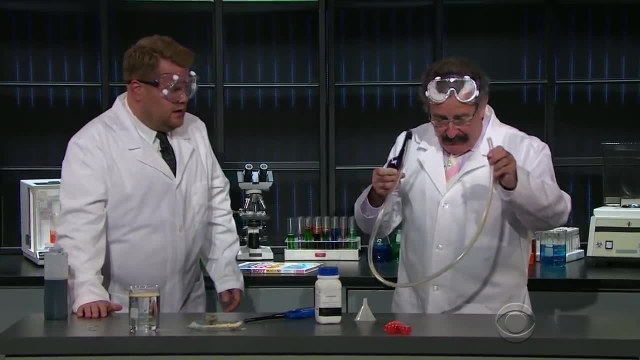 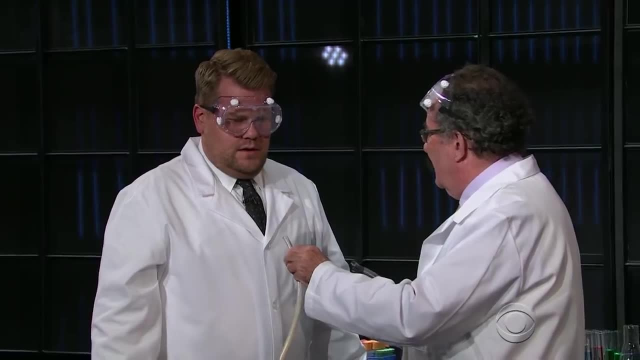 I've got some lycopodium powder in this tube. OK, I want you to be, absolutely. You must promise me, Yes, that you'll blow into this tube and not suck it LAUGHTER. Sure, yeah, So hold it like that. 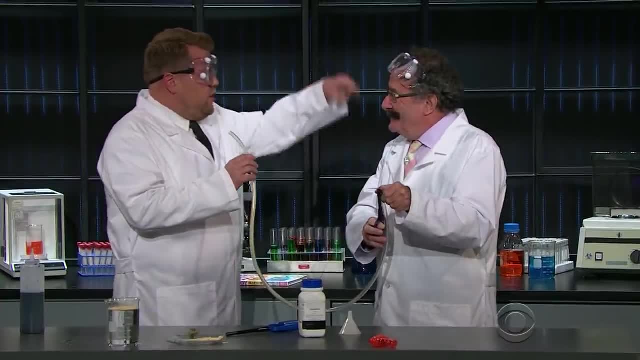 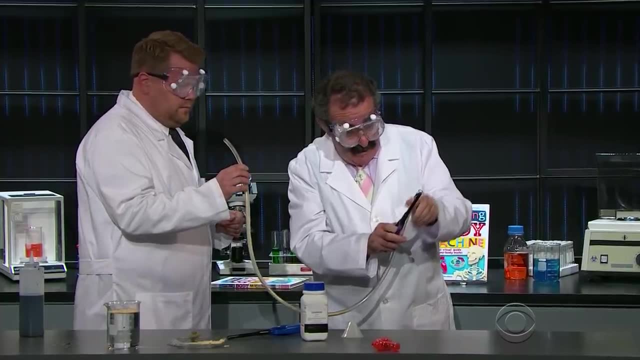 I've done this at the side of the road before LAUGHTER. Put your goggles on. OK, Right now, All right, So well, I'm going to light this thing, Yeah, and you're going to blow not too hard, fairly continuously, gently. 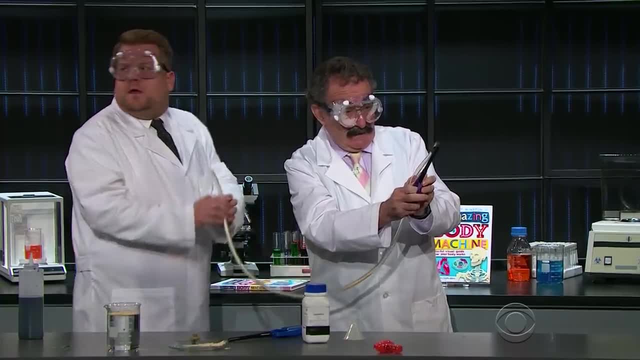 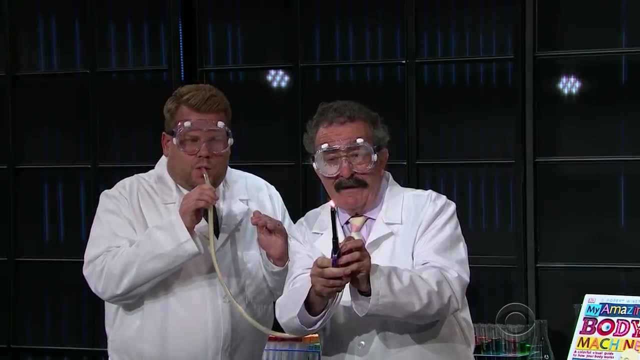 and I'm going to try and set the whole theatre on fire. LAUGHTER, Wait, wait, wait, don't do it until I tell you, Don't worry, I'm in no rush. Go, BELL RINGS, CHEERING AND APPLAUSE. 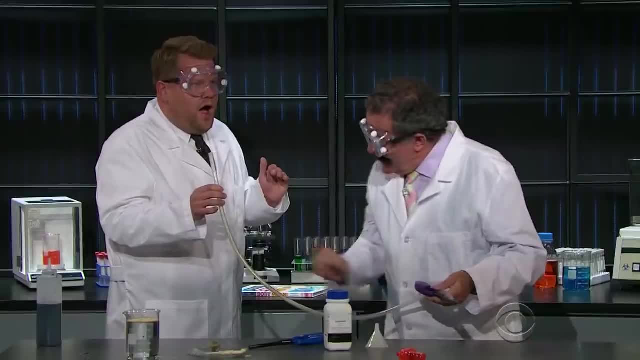 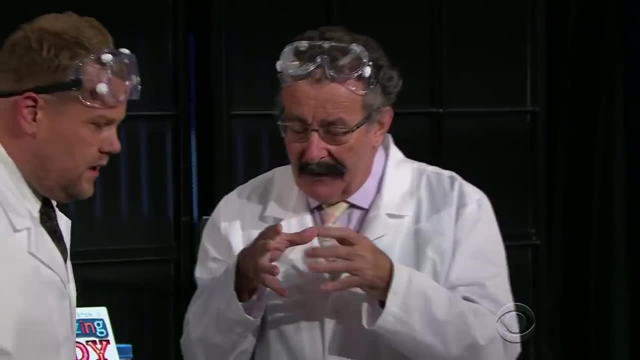 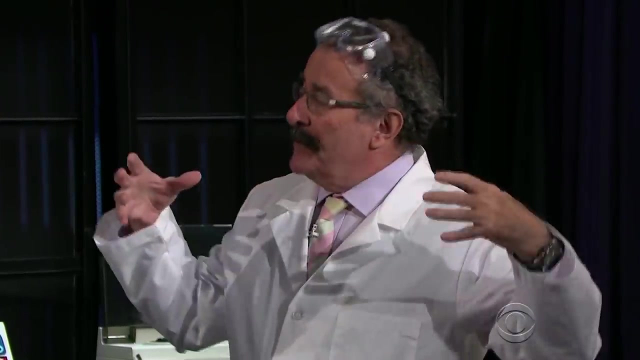 APPLAUSE. So basically, CHEERING AND APPLAUSE. That works because those particles, those little seeds, are full of fat, Yeah, And that fat ignites. And when the particles are mixing with oxygen in the air separated from each other, they can oxidise, they can burn. 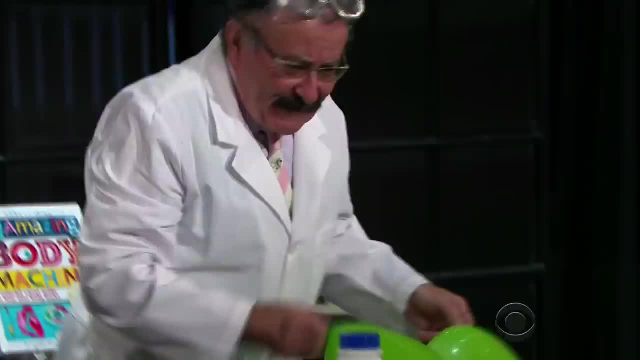 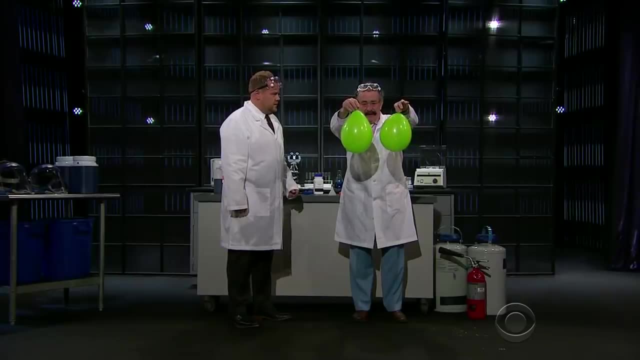 That's amazing. That's how it works. What have you got for us now, Rob? What's happening here? What have we got here? Come on the front, OK, All right, Watch these two balloons. OK, One's been blown up with ordinary air. 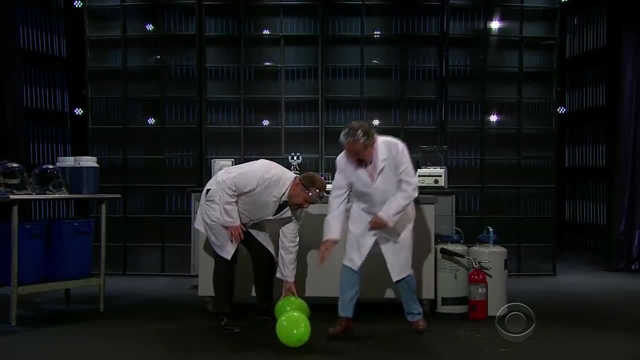 And what's in that one? That one's really heavy, isn't it? Yes, it is. Pick it up and see how heavy it is. So what's in there? It is sulphur hexafluoride. OK. 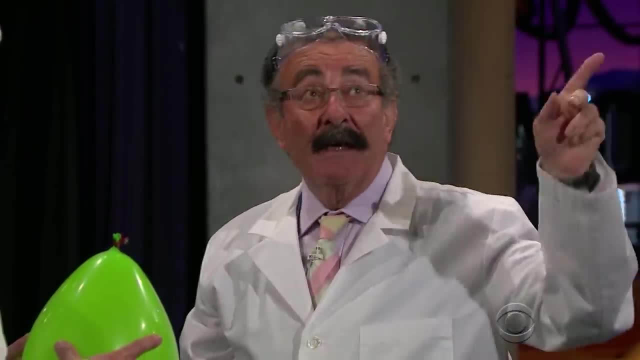 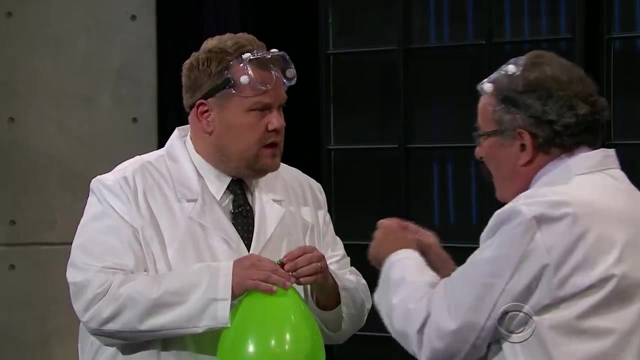 Which is one of the heaviest gases available. It's about six times heavier than atmospheric air. Right, What I want you to do, because it's a very, very dense gas? Yeah, but not until I tell you OK. 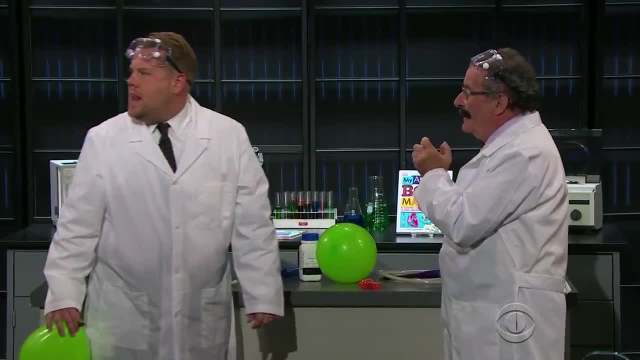 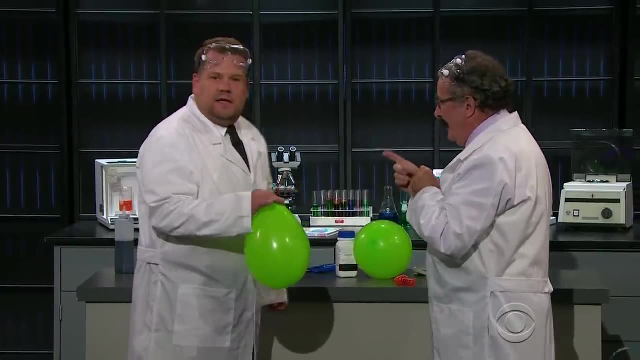 I want you to inhale it LAUGHTER, And then I don't think it's that sort of balloon, Reg. Go on, You want me to inhale it. I want you to inhale it, but you mustn't inhale too much of it, because it'll fill your lung. 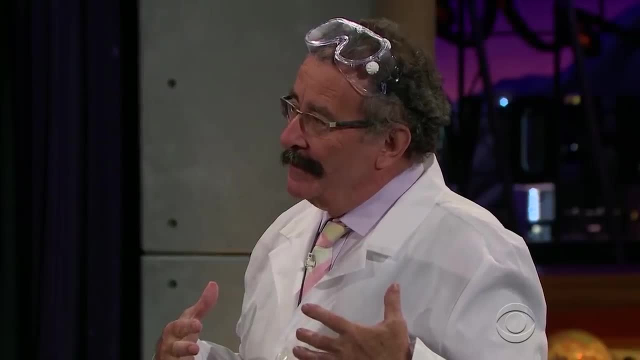 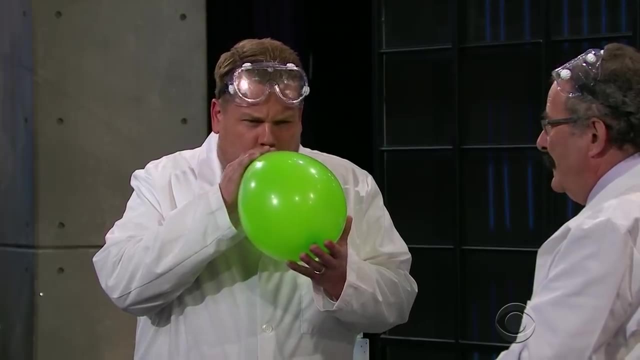 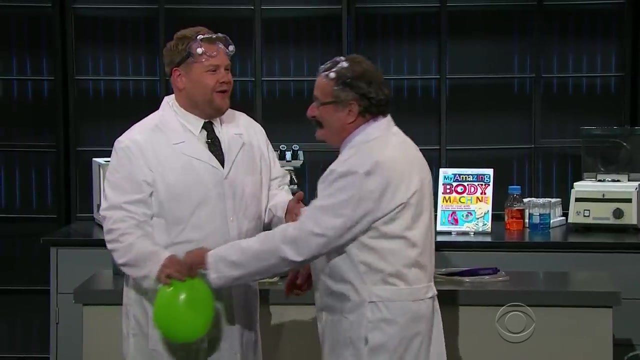 And it'll displace all the oxygen, and that might be a bit sad really. So All right, OK, hang on. That's enough, OK. Oh my God LAUGHTER. Oh my God, That's ridiculous. 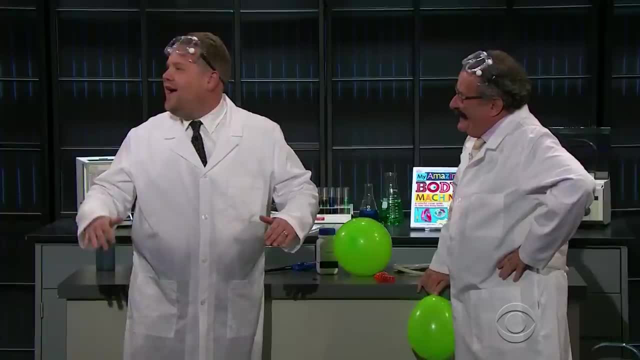 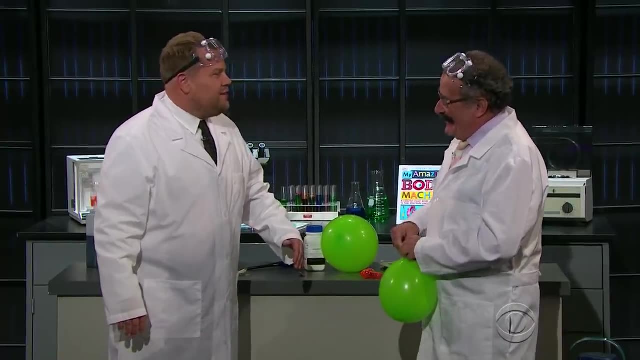 I'm not even putting your voice on. that's why, LAUGHTER, I sound like the start of the Run so hard. LAUGHTER, Breathe that. Come on, cough, Breathe that. What do you mean, cough? How long will it stay like this? 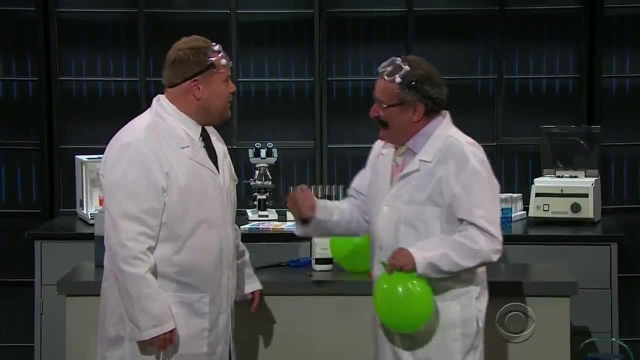 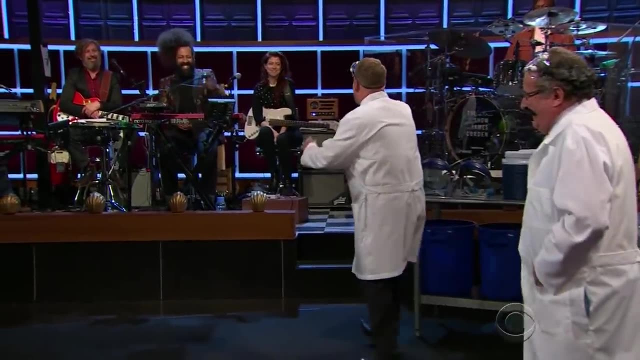 How long will it stay like this? When does it Breathe? When will it come back? Give it to Reggie. His voice is: Are you going to do some, Reg, Are you OK? Go on, OK, Go on. 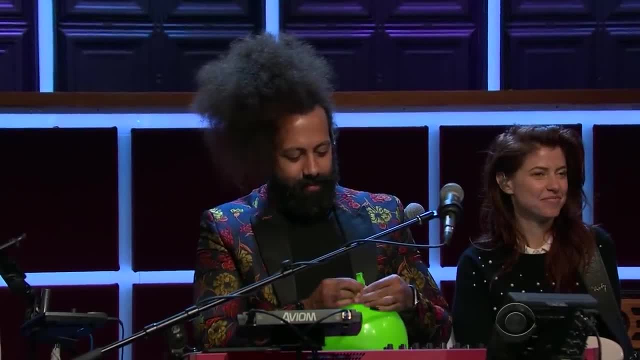 OK, Ah Ha, I feel like mine's coming back. Has it come back or is it? Have I got used to it? Is it back? All right, let's go, Reg, Here we go, Not too much. 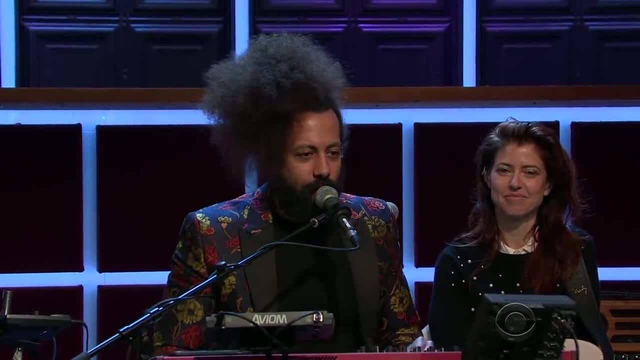 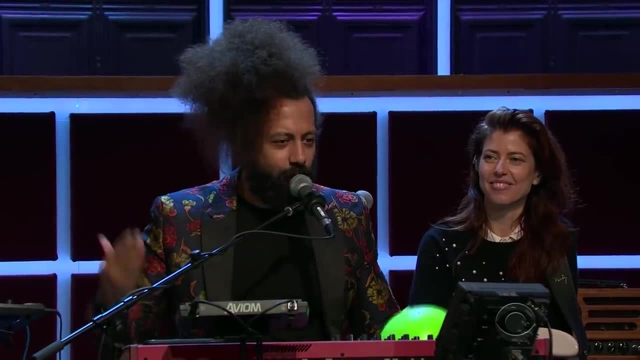 LAUGHTER, LAUGHTER, LAUGHTER. I feel like my body's got to go down to the store buy some cabbages. Everybody needs a little cabbages. what You know, it's like inhaling Freon LAUGHTER. 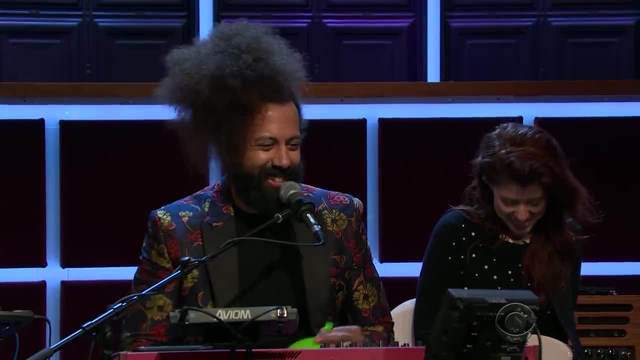 You know what I feel like putting lotion in the basket, James. we'd better move on, All right, All right, what's next? What's next, Robert? What are we doing? I think we're going to wear some protective gear. 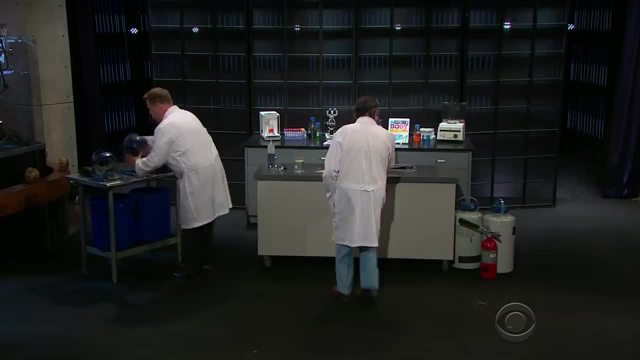 Would you like to put the helmets on? Yes, absolutely OK. Hand me the other one. OK, here we go. There's your helmet, And wait, you've got to have some gloves as well. There's gloves here as well. That would be a very good idea. 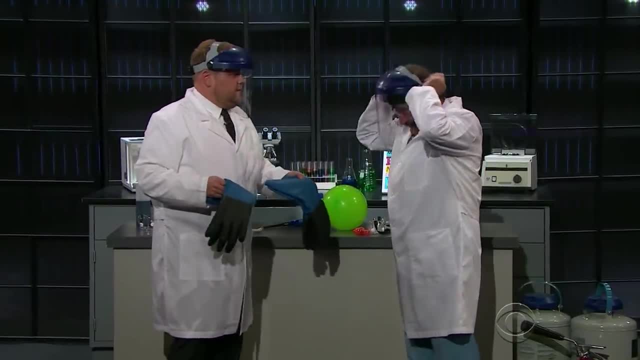 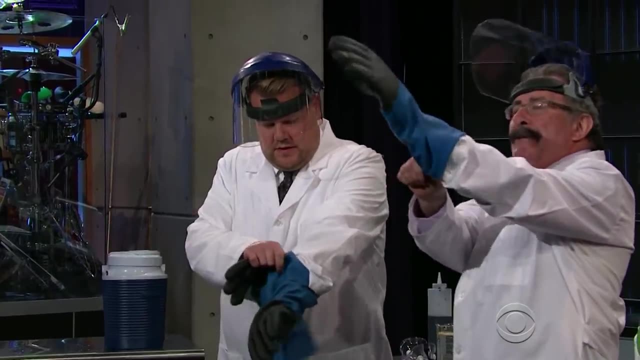 OK, That's it. There you go. I've got it There, you are Right, OK. OK, I'm always slightly worried when you come down and we make us put gloves on, because Last time you poured liquid nitrogen all over my genitals. I remember. 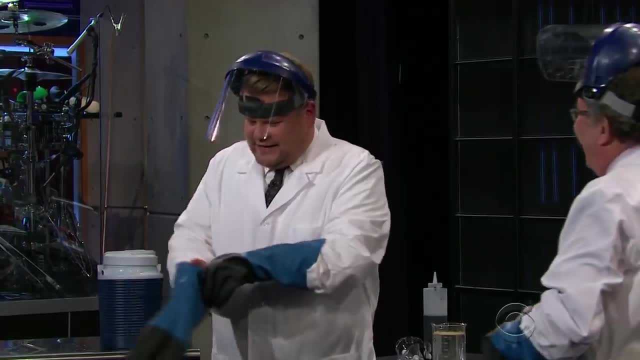 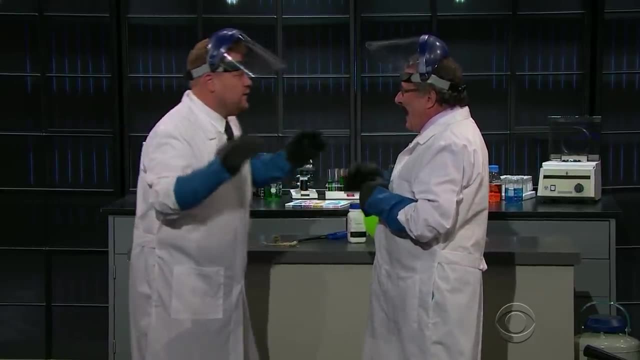 LAUGHTER. Yeah, and I feel like today's experiment has just been one long. You trying to get back at me for that moment. I didn't do it on purpose, OK, so what are we doing? You've got some blue bins there, The ones on the bottom. 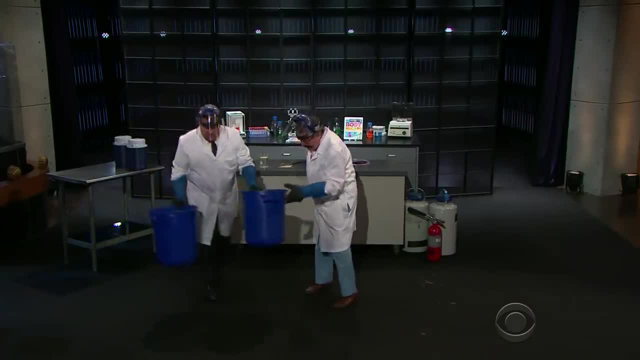 Yep, OK, You put one there and I'll take it. OK, Yeah, it'll do fine. All right, Right Now I've got some liquid nitrogen, quite a lot of it. OK, Oh, One each, is it? 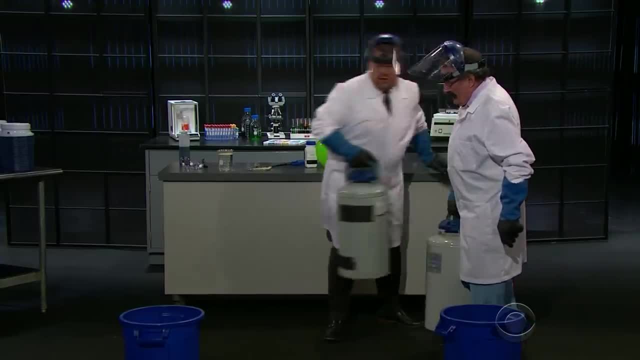 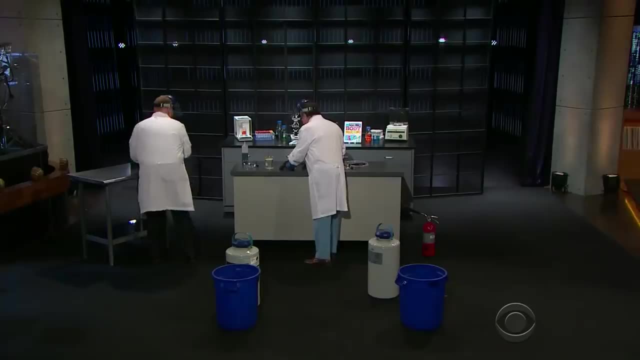 Shall, I take this one. Yeah, OK And OK. And before we pour it in there: Yeah, we're going to put these on the bench. OK, Just put them here. so we're at hand. And what's in here? 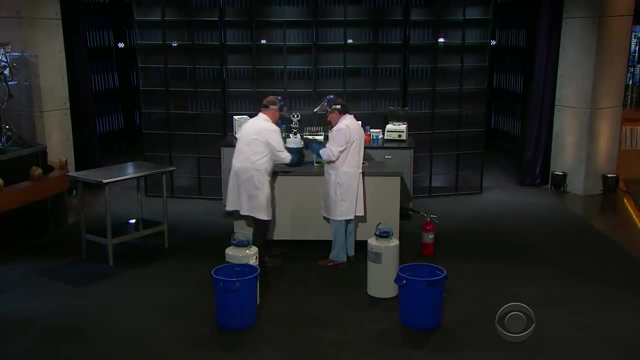 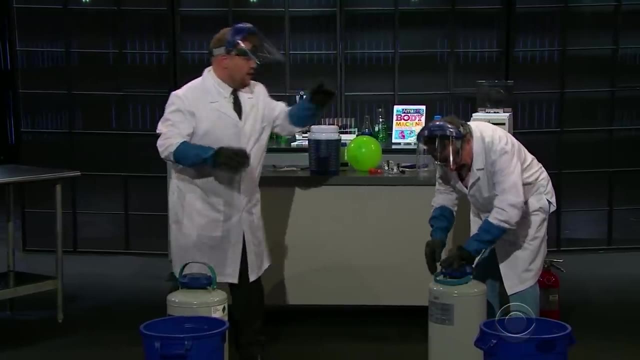 Well, It already feels dangerous. Not a lot, OK. so What are we actually trying to do here, Robert? What are we aiming for? We're going to take the liquid nitrogen and we're going to Hang on. I feel like this is when we need these down, is it? 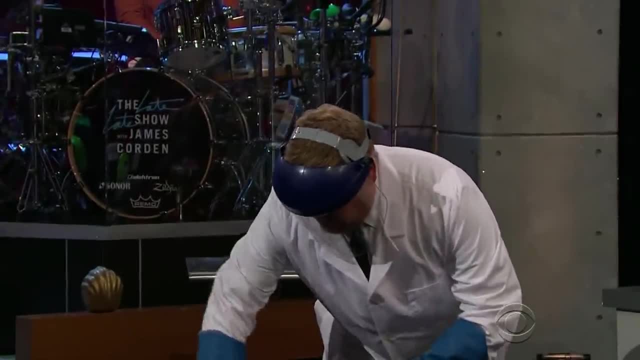 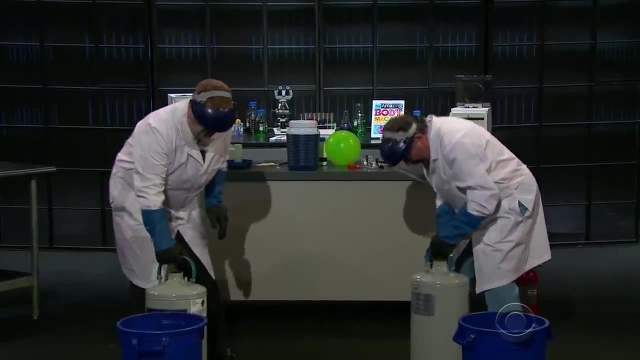 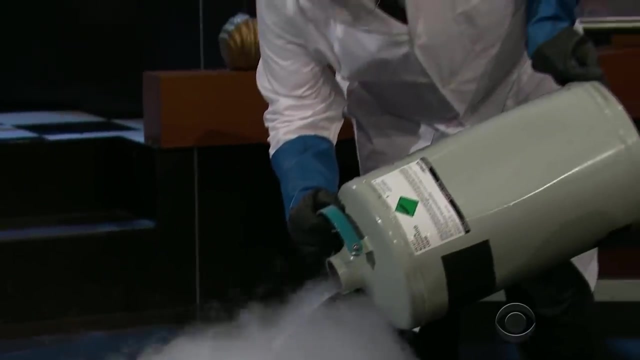 We will in a sec. OK, Right, I feel like I'm in Breaking Bad. Now And now what? Take your liquid nitrogen, Yes, and pour it rapidly into the blue thing In here. Yep, Ooh, How much? As much as you can. 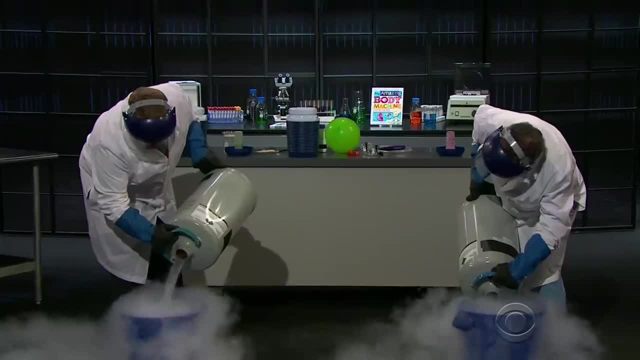 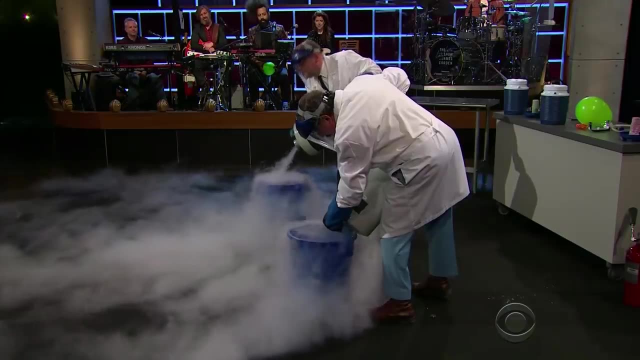 OK, The lot. Well, I can't really see the top, so It really is like a guesstimate. Try not to get it on your shoes. OK, thanks for telling me that, just as I get to the bottom of it.